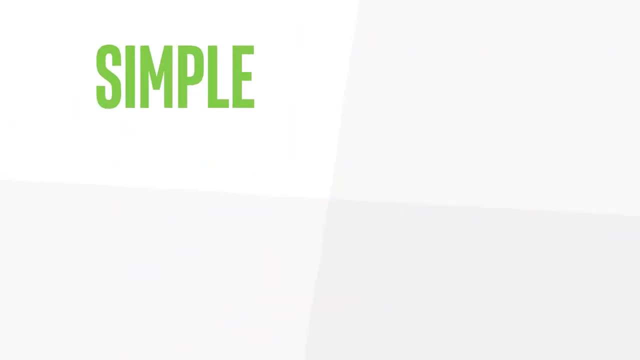 glucose and vitamin D. Carbohydrates are macronutrients that supply energy to the body in the form of glucose and vitamin D And raise blood glucose levels. They can be simple, which increase blood glucose levels rapidly, or complex, which increase blood. 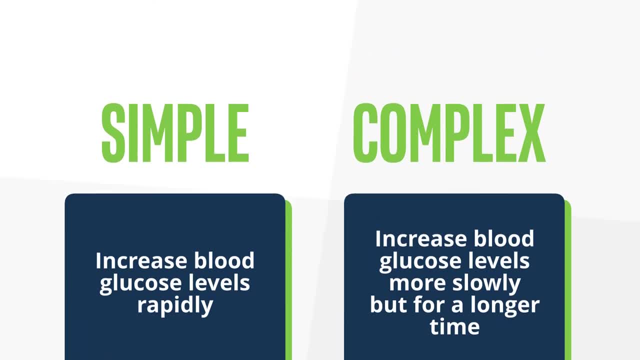 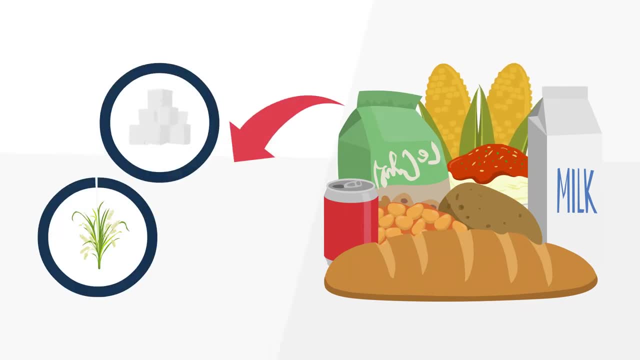 glucose levels more slowly but for a longer time, and they are found in a wide array of both healthy and unhealthy foods. They also come in a variety of forms like sugars, fibers and starches. Protein can also be a source of energy for the body. 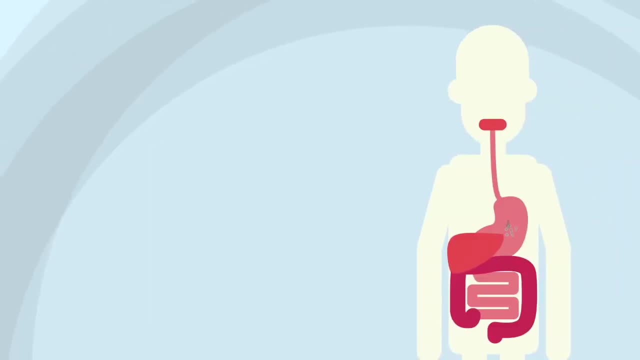 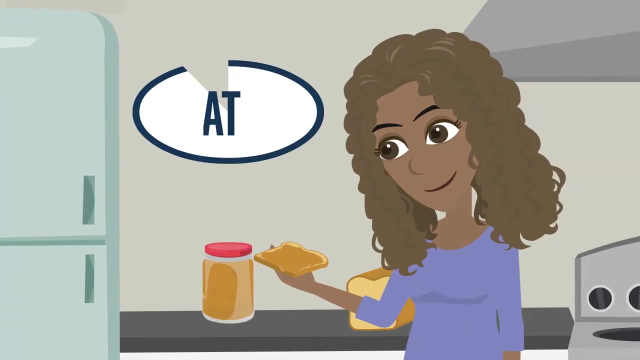 During digestion, proteins are broken down into peptides and amino acids, which are then used for tissue maintenance, replacement, function and growth. If the body is not getting enough calories from dietary sources or tissue stores, protein may be used for energy. Fat is another important macronutrient. 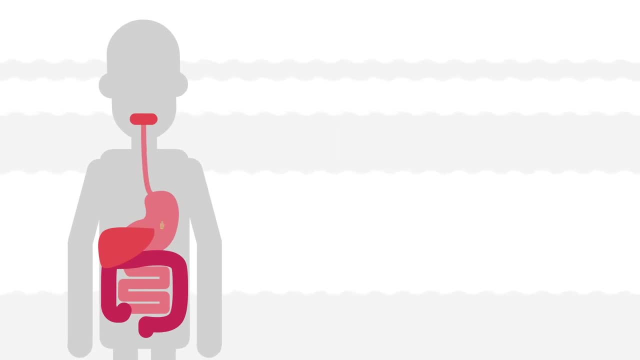 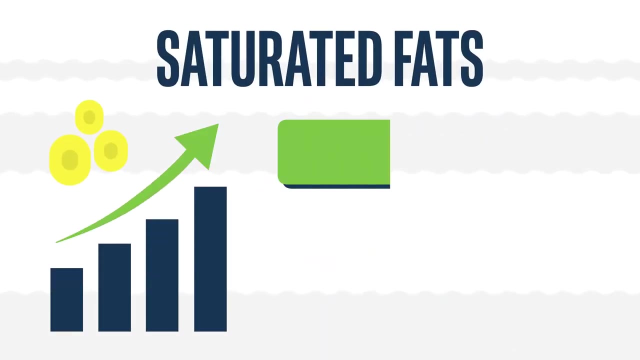 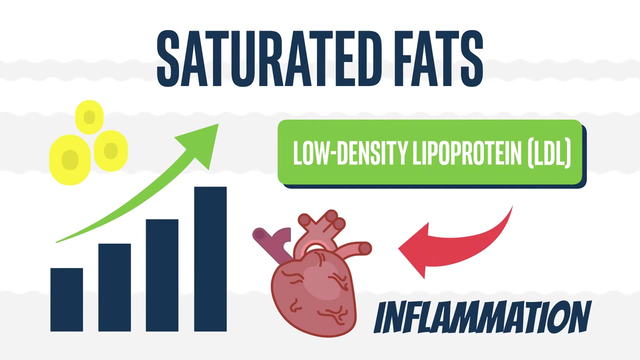 During digestion, fats are broken down into fatty acids and glycerol, which are required for tissue growth and hormone production. Saturated fats raise blood lipids, including low-density lipoprotein cholesterol levels, and certain other heart disease risk factors such as inflammation. 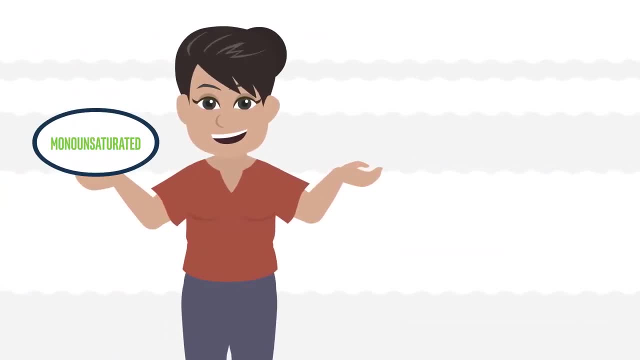 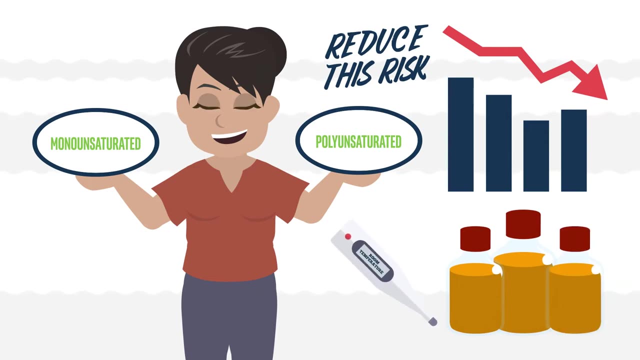 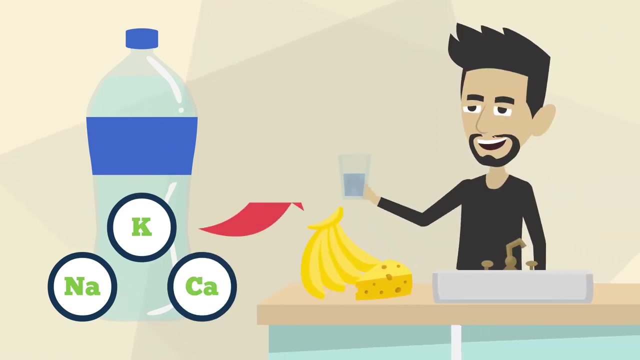 Some evidence suggests that choosing monounsaturated and polyunsaturated fats in place of saturated fat may reduce this risk. These fats are liquid at room temperature. Water and macrominerals such as sodium, potassium and calcium are the other types of macronutrients that should make up a significant part of a healthy diet. 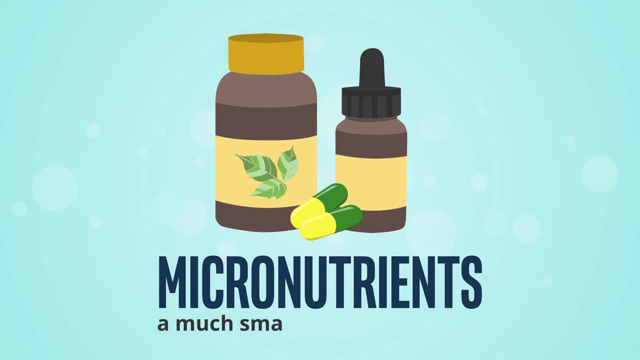 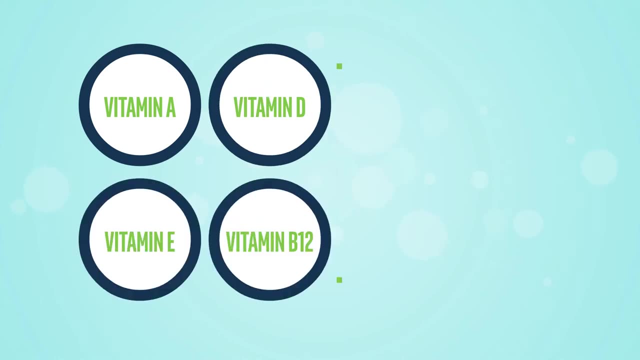 The vitamins and minerals considered micronutrients should take up a much smaller part of our diet than the macronutrients. Only vitamins A, D, E and B12 are stored to any significant extent in the body. The other vitamins referred to as essential vitamins. 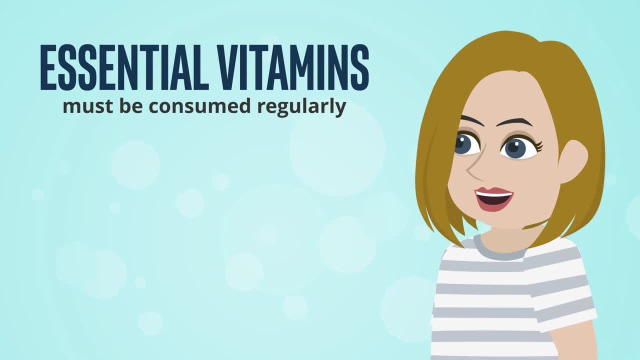 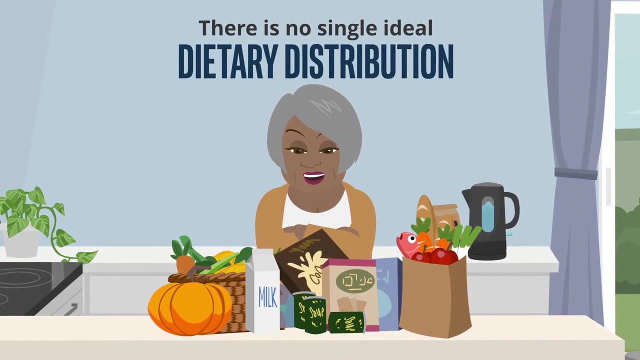 must be consumed regularly to maintain tissue health. Essential trace minerals include chromium, copper, iodine, iron, manganese, molybdenum, selenium and zinc. For patients with diabetes, there is no single ideal dietary district. The most important thing is the proper distribution of calories among carbohydrates, fats and proteins. 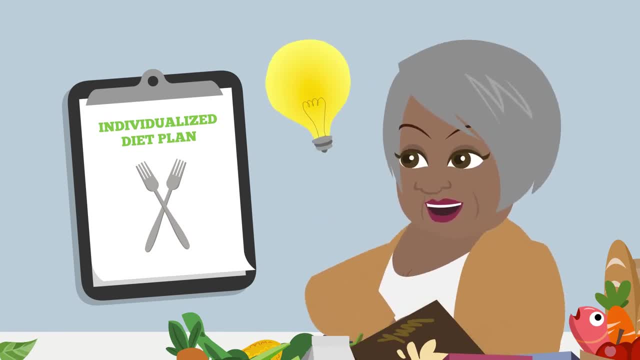 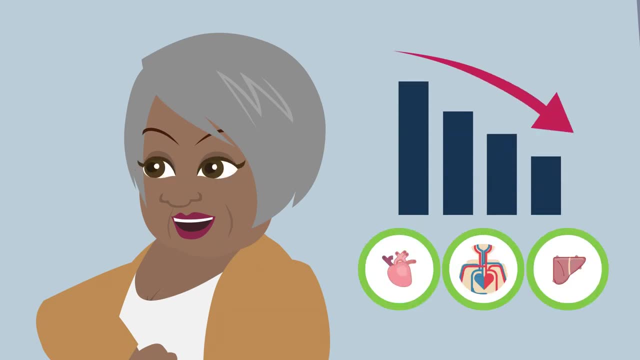 Rather, dietary plans must be individualized, keeping total caloric and metabolic goals in mind and reducing risk for cardiovascular disease, microvascular diseases and fatty liver disease.